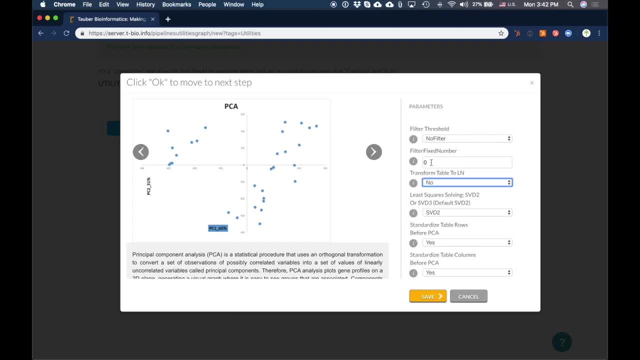 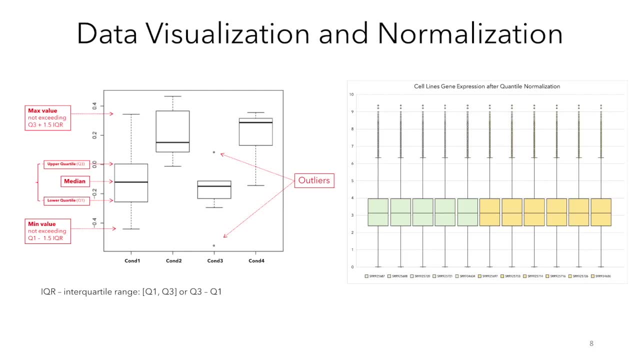 For example, we will cover different visualization and normalization techniques. how do we leverage the visual information that we have in these methods and how do we understand the application of these types of visualization techniques to help us understand the data that we're dealing with? 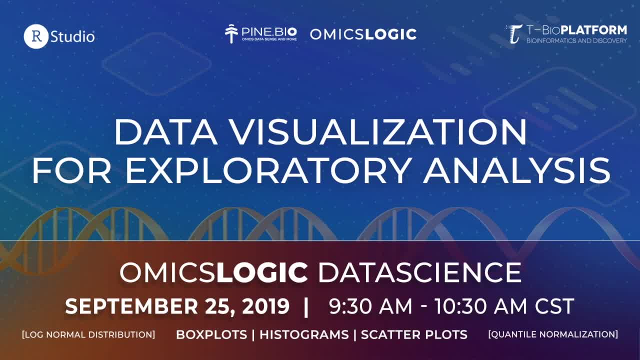 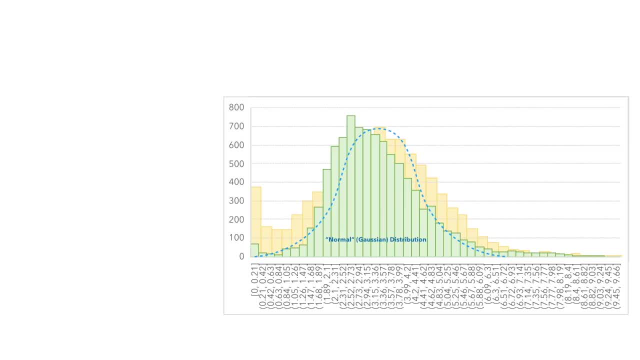 Later on we will talk about other types of exploratory data analysis tools and other types of digital visualizations. We will, for example, talk about distribution of data to find correlations between different replicates. so we'll talk about what part of it is technical noise, what part of it contains actual G-Expression. 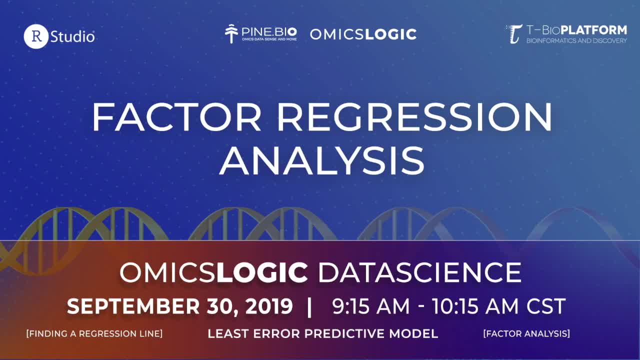 And then I'll talk about how to use regression to spot new and more complex trends. So we'll talk about how to use the speaker to determine a more orientational and resource-rich database of data in the future, to make sure data can be used for learning. 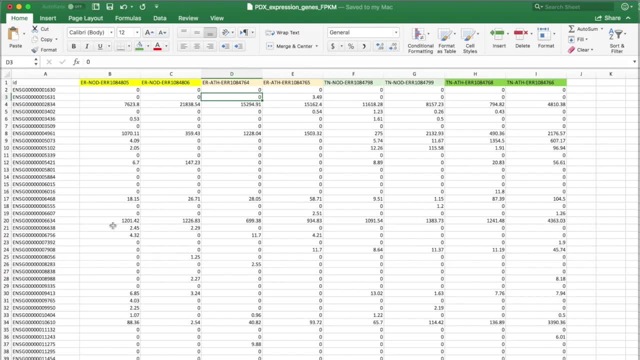 And now we'll be talking about new methodsJAEM, file processing and our vino對啊z וא�. the specialized stage of data, and new protectors and eighty racing data, rę command, the regression to spot complex trends that go beyond just a comparison of two different conditions. 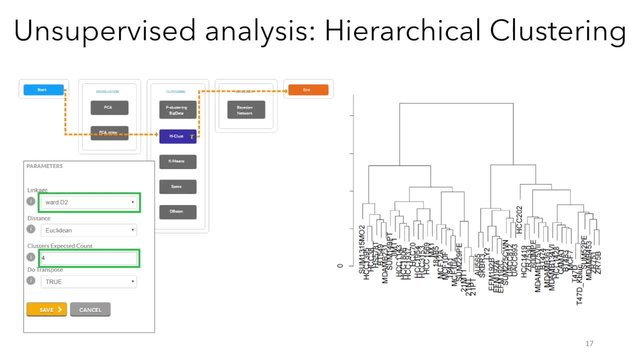 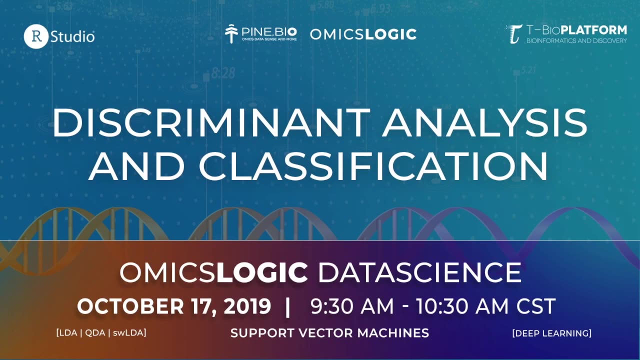 and move on to clusters: how to understand the different linkage methods, distances and how to understand the relationships between clusters, as well as a variety of different types of clustering methods. the omics logic training program will cover a variety of methods for high throughput data processing. analysis and visualization will help you apply these methods to clinical 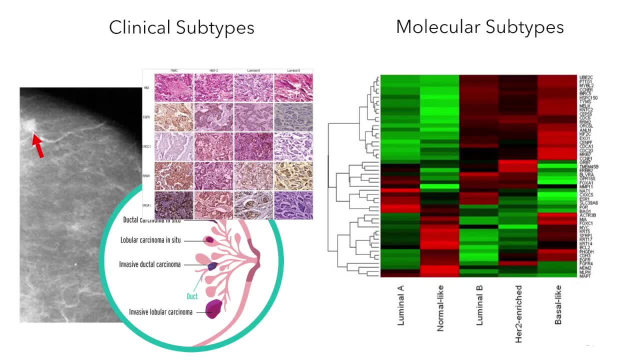 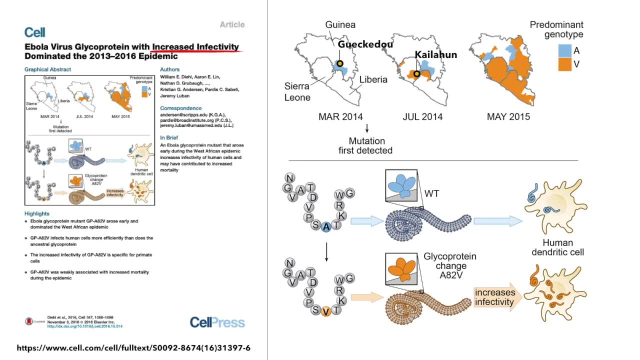 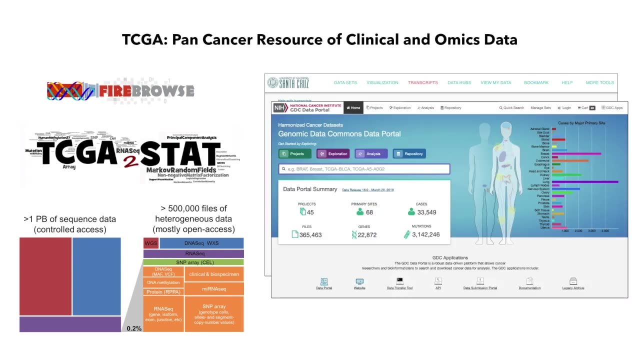 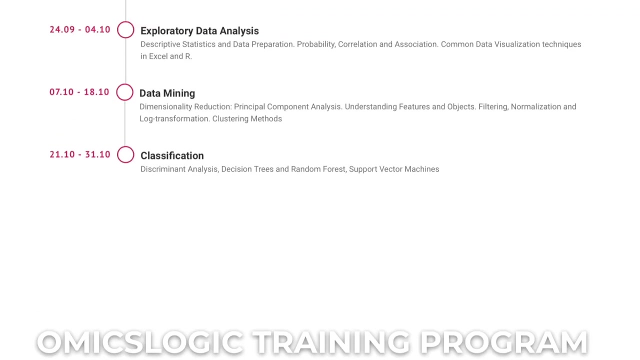 research and pharmaceutical projects will prepare you and help you design and plan the analysis to make it impactful, build up your portfolio of projects and analysis examples, understand biomedical research and read publications critically. and finally, you'll be able to obtain a certificate of completion. to improve your city, the program will provide you with a variety of 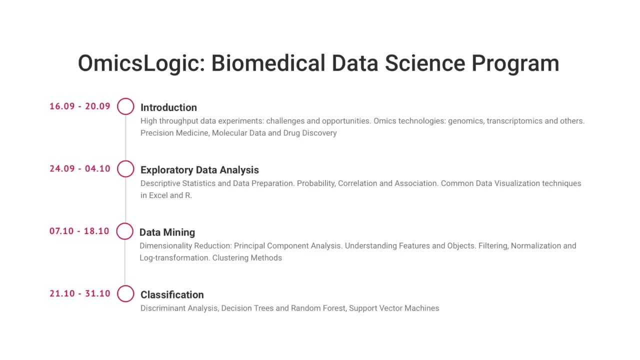 tools and resources to help you develop your own research and analysis. program itself will spend two months of hands-on training, where you will meet twice a week to discuss these different methods and projects, and then another month and a half to spend on your own project preparing the analysis. 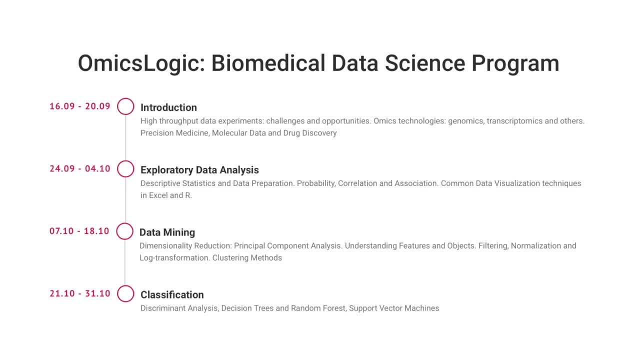 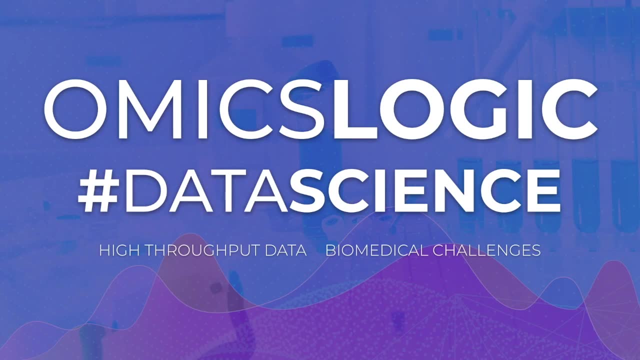 designing the analysis and being ready to apply the skills that you've obtained throughout the program to a data set of zero. you